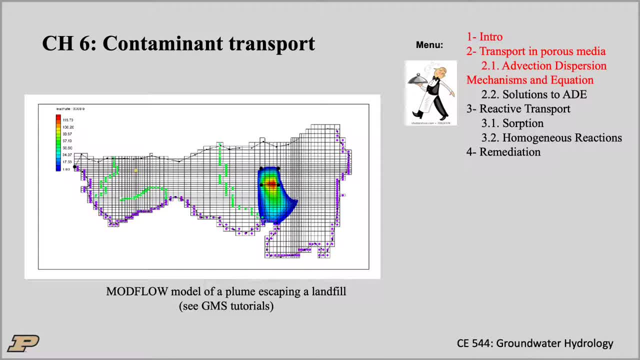 for the chapter and introduce transport transport equations. so advection, dispersion, the mechanisms linked to it and then the equations that we use to describe transport. In the next lecture I'll go through solutions and examples And then after that we'll get. 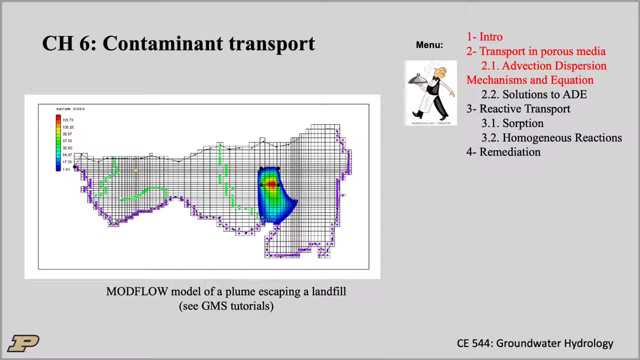 into reactive transport And more specifically, we'll study sorption first and then homogeneity reactions and finally, the last lecture will be on remediation. so what do we do when there is contaminant in the groundwater? basically, here you can see on the left hand side, on the left hand side, here that GMS model that you have. 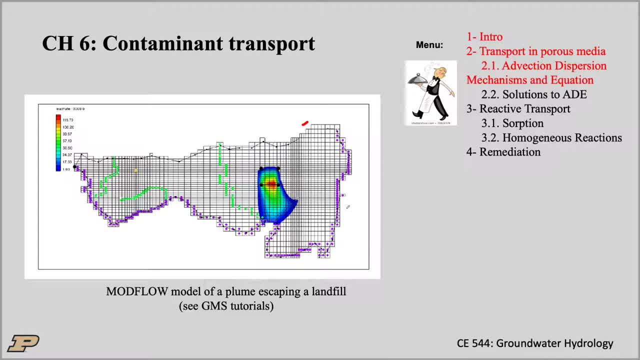 to do for Friday. so this is you know the tutorial that you'll do for Friday. so you can see, here we have a landfill that is leaching into the aquifer and you can see the plume spreading out of the landfill into. you know the domain. so 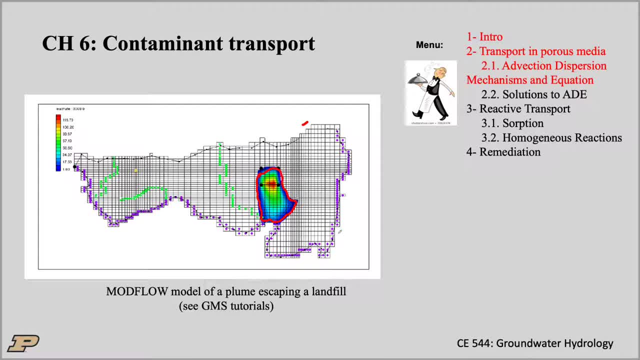 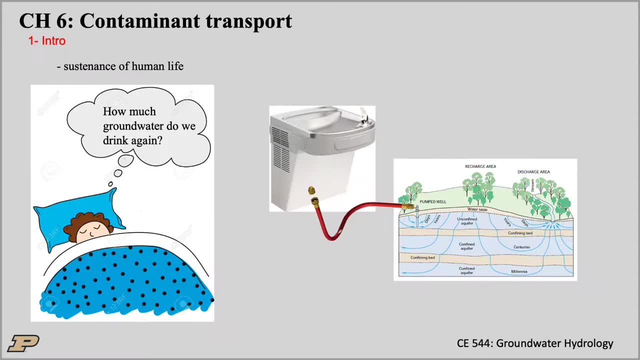 we. that's basically. what we'll be studying is how those processes work and how we actually model. so what's behind? if you will, the GMS simulations here, okay, so let's start with the intro and again dreaming about your groundwater class. if you remember the intro, you can see that the GMS simulation is actually. 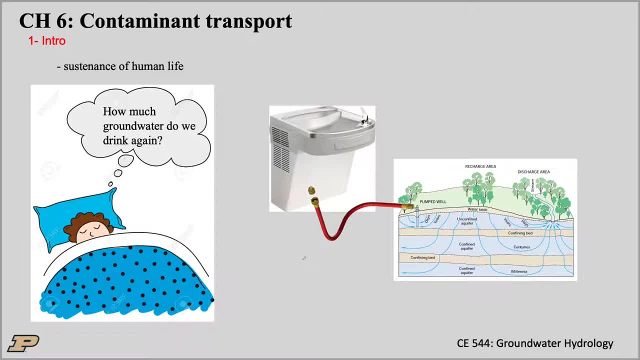 there, right so, if you remember from chapter one. so now we're really jumping back to the first lectures in this course. how much groundwater do we drink? again, right? so how much groundwater do we drink? why do we care? you've got what is contaminated. well, mostly because we use ground water. and more specifically, 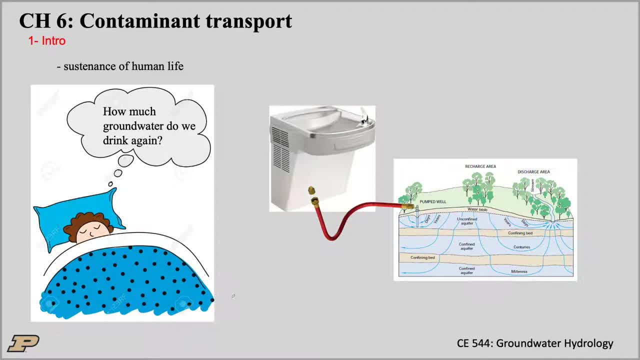 because we drink it right. so that's a problem if there is pollution in there. again you can see here there's a pump right pumping some groundwater for or maybe a house, and then you know that goes directly to your fountain here. So again, we don't want contamination in this water. 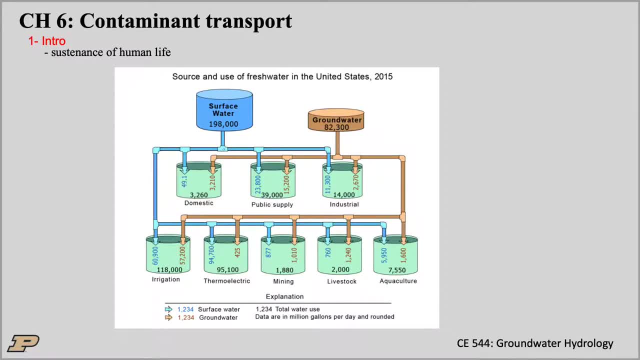 And again, to answer that question, specifically what we want to focus on for today, right, I'm not going to go through this whole thing again, but you'll recognize this plot from Chapter 1.. And here the part that I'm highlighting right is the domestic and public supply of. 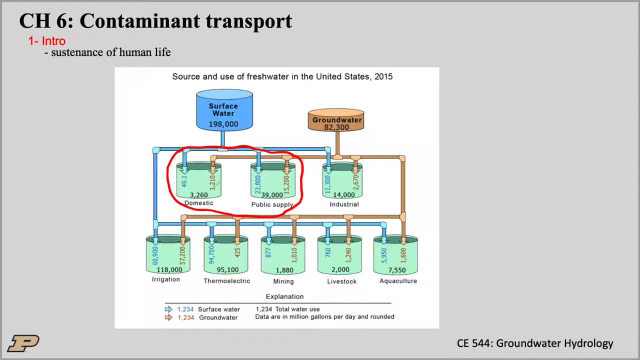 drinking water And you can see, for domestic supply, groundwater is overwhelming. the overwhelming source, right Again, individuals have wells. You know, if you're not connected to public supplies, basically you have a well and that's groundwater, Even the public supplies. you can see here there's a bit more surface water than groundwater. 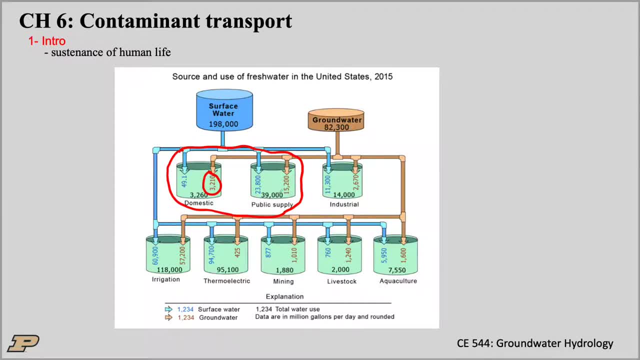 but we're not that far from 50-50, maybe like 40-60 or something. So, again, a lot of groundwater is used for drinking and we want that water to be pure, right, Right Drinking, Drinking quality. 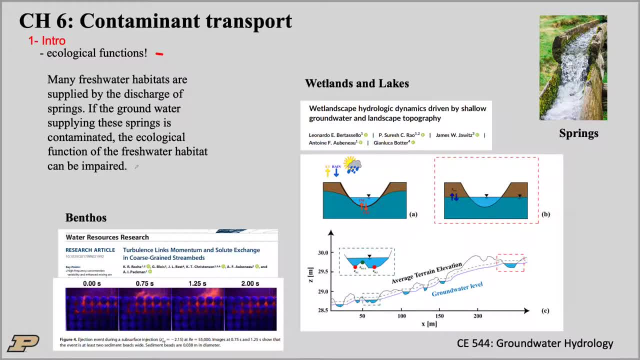 So, beyond this sustenance aspect of groundwater- right, we need groundwater to drink. We Groundwater is also important for ecological functions, right? So many habitats are supplied by the discharge of groundwater into surface waters or even groundwater. habitats themselves are important. 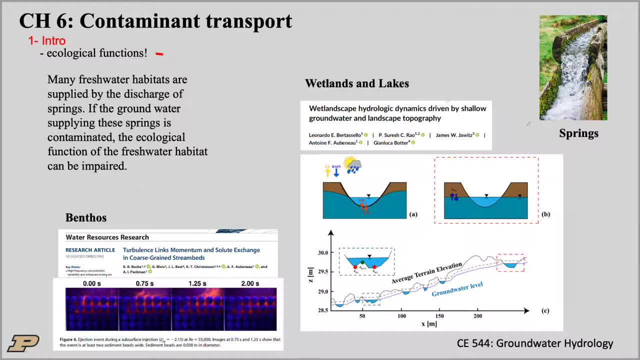 So I just put a few examples here. So on the top right, the springs right. So this is literally, you know, groundwater coming out of the floor of the ground and feeding some habitat, So all the spring habitats you can think of. you know, we want those to remain pristine. 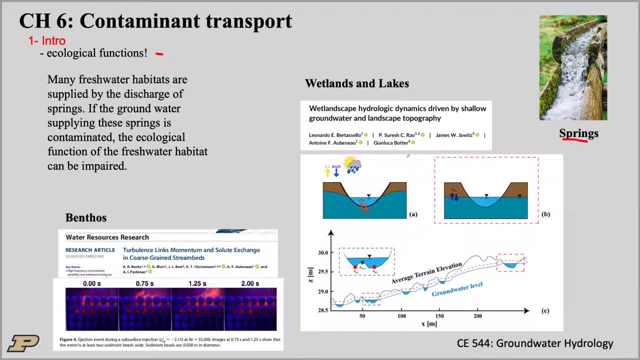 Of course, here, wetlands and lakes, and these are a couple examples. You notice that these two papers that I put here are, you know, my papers. And here's a study where we looked at the influence of groundwater on wetlands and 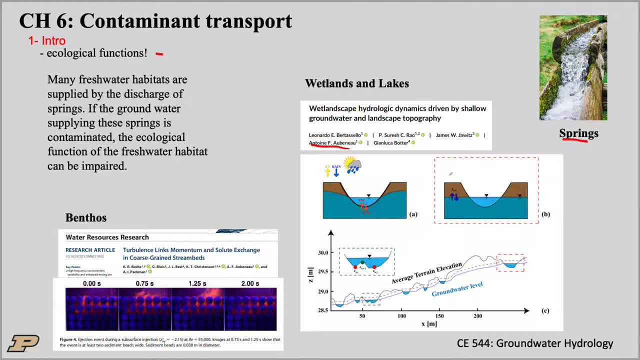 you know the Hydroecological functions of wetlands. So my former students, Leonardo spent his whole PhD thinking of those issues, basically both on the hydrology side and on the ecological side. So hydroecological side. 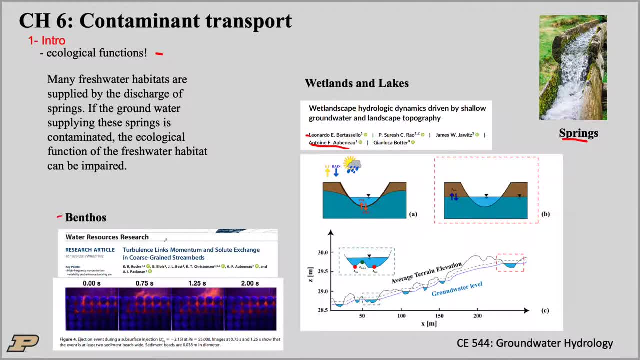 Another habitat that people don't really think about much is the benthos, right? So benthos is that bottom of river, So if you imagine, this is the porous media down here, right? So this is below the water and then this is the surface water up here. 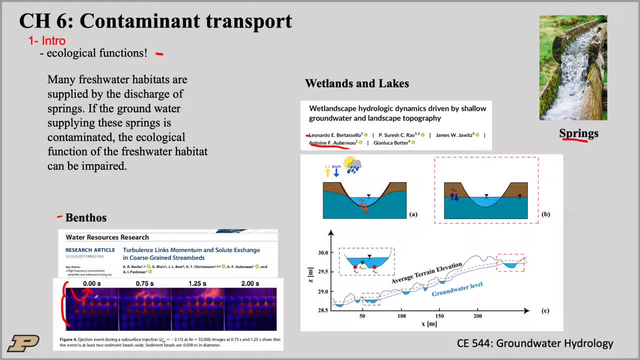 There is exchange of water between the surface and the subsurface and, of course, at the bottom of the river, right here is where all the algae and biofilm live, right. So you can see, here there's a lot of exchange. 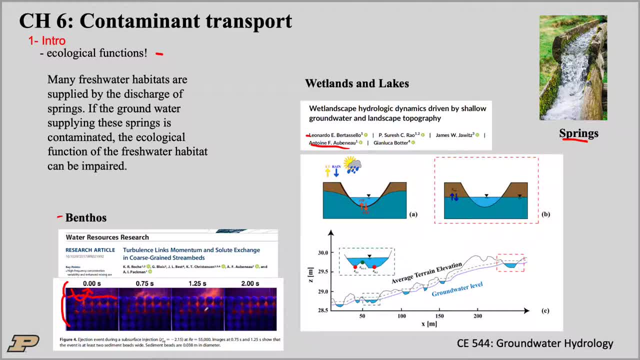 You know, you can see that plume of rhodamine. This is a dye, So there's water going, you know, from the surface to the subsurface and back And again, if there's pollution coming from the original groundwater into this zone here. 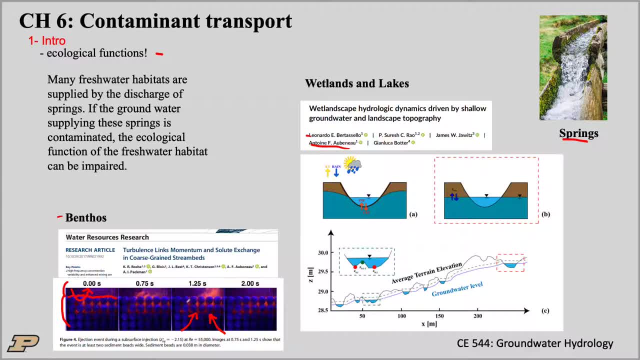 then you know this whole interface is polluted And this is a very important interface for biogeochemical functioning, like nitrate, phosphate, cycling, etc. carbon. So very, very important habitats at the bottom of rivers. Okay. 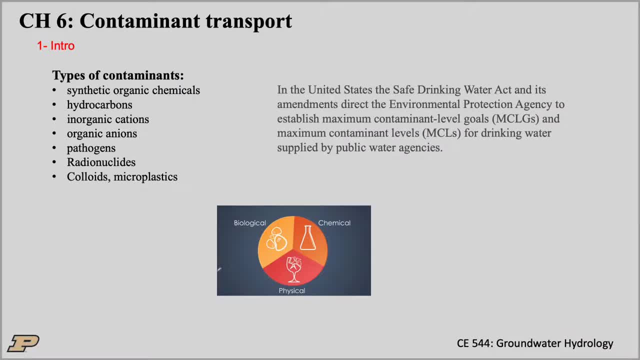 So a list of types of contaminants- And there are many. We won't see them all, obviously, But there's many, many different kinds of contaminants you can find in groundwater. So organic chemicals are a big problem. They bioaccumulate. 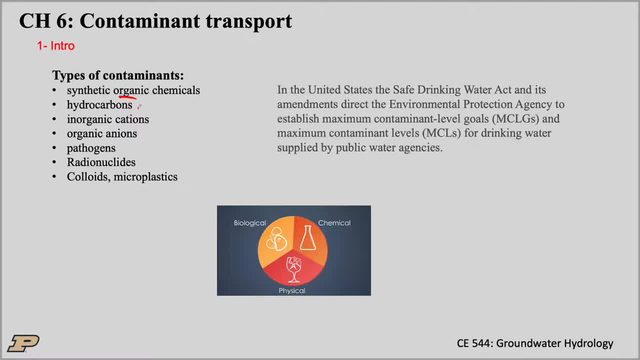 You know They're, Some of them, very nasty. Hydrocarbons are obvious. You know, organic cation and organic anion, So ions and metals and those kinds of things, Some pathogens. So there's, you know, lots of issues with, say, E coli pollution or cryptosporidium. 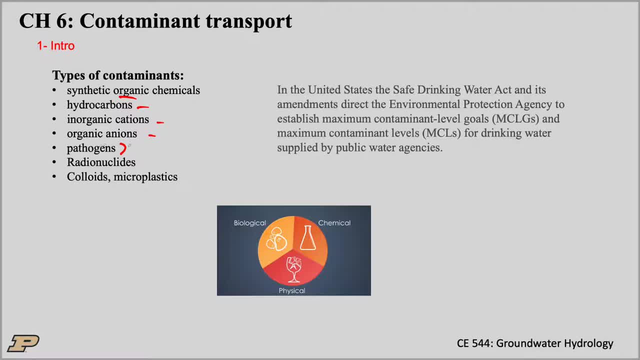 I also have a couple papers on that. So transport of pathogens basically in groundwater and then, maybe, you know, contaminating some surface water or drinking water Or drinking water wells, etc. Radioactivity- obviously we don't want that in the groundwater. 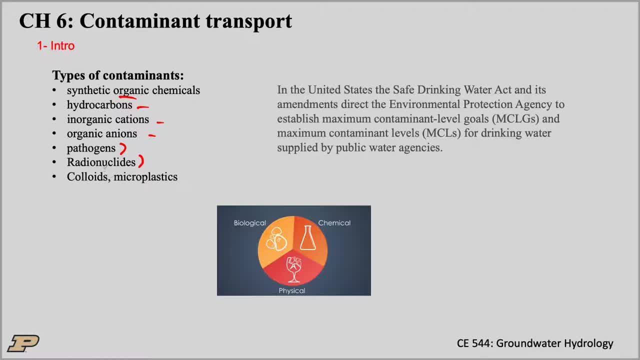 There's plenty of issues down in Oak Ridge where the original, you know atomic experiments were conducted. There's tons of storage down there and you know a lot of pollution of groundwater by radioactive materials And then finally colloids. 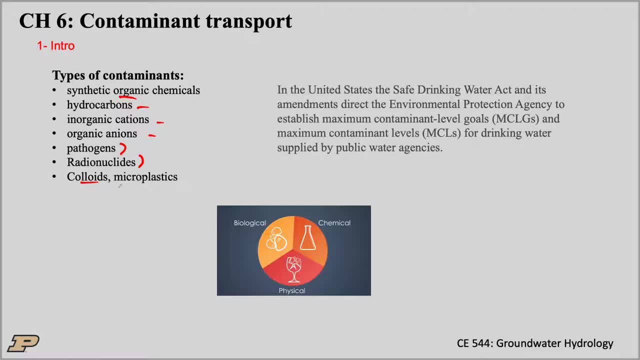 So colloids are like solids, basically Little particles that can infiltrate. For example, a modern, you know issue is microplastics. Those plastics that deteriorate create little microparticles and then those things you know are found are pervasive, basically in the environment, including groundwater. 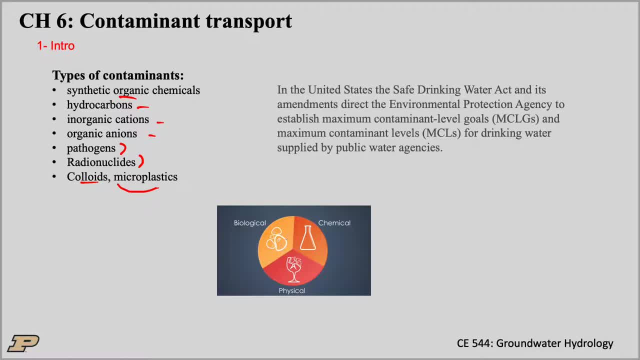 Just a quick sketch here. I can't remember the source of this. I should have put the source, But in general right, the broad categories are chemical, biological and physical contaminants And you can see the link here on the left to that list, to this graph here. 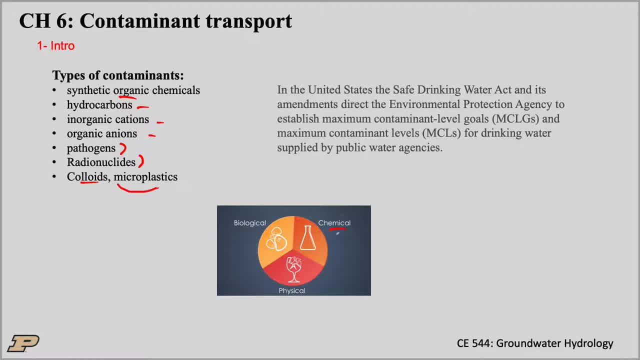 So for this course- you know this chapter- mostly we'll talk about chemical reactions and chemical pollutions And we'll talk a little bit about colloids towards the end. And colloids can be, you know, biological, so pathogens, you know cells, or they can. 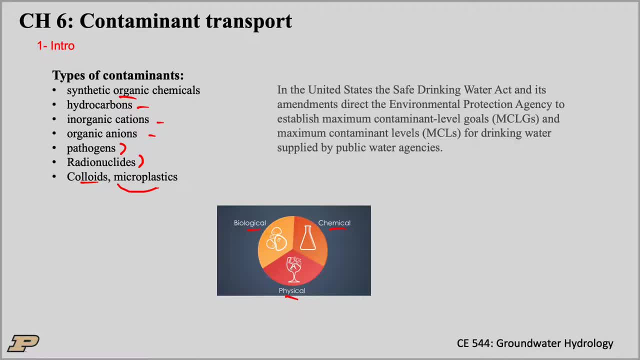 be physical, like I said, microplastics and stuff. So filtering and all that stuff is more on that biological physical pollution. But most of the chapter will be on chemical pollutants And here I put again an excerpt of Fetter. 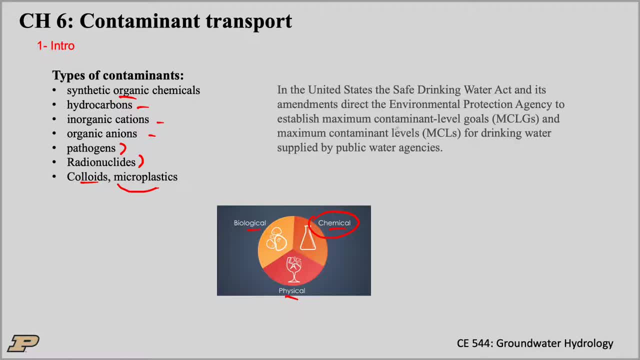 So we have that Safe Drinking Water Act. I think that's from the 80s- actually pretty late or pretty recent, I guess you could say. But we do have maximum contaminant levels, So a lot of those pollutants are controlled or, you know, there's legislation for a lot of them. 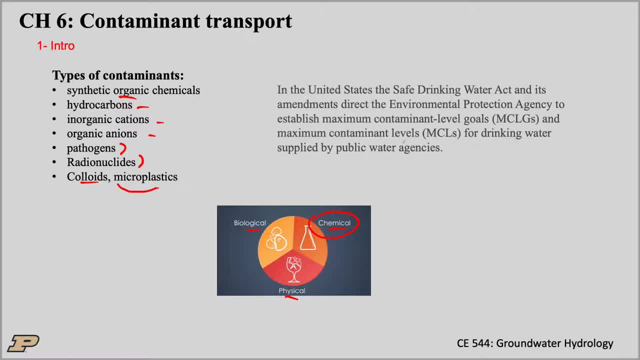 So there's a maximum contaminant level for drinking water supplies, right that need to be respected, And then there's goals that are not really enforced, but you know, some compounds have, you know, zero goal, for example. 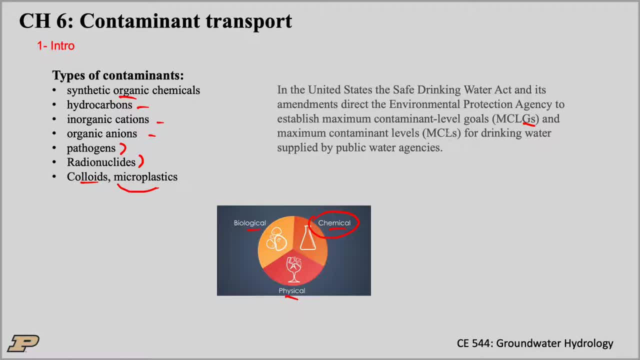 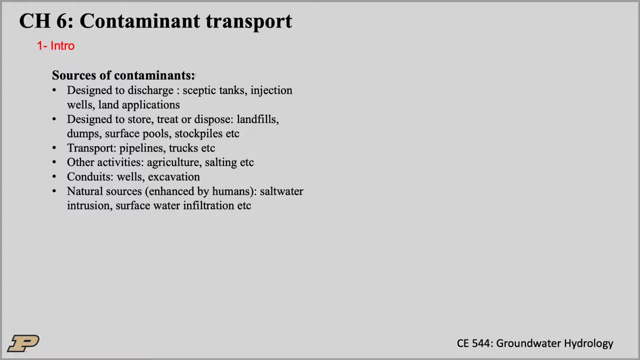 But then the maximum possible is, you know, whatever that number is. So all contaminants. basically, you can look up the EPA website and find their allowable concentrations. Okay, another aspect. So this was a list of different contaminants. Here's a list of their sources. 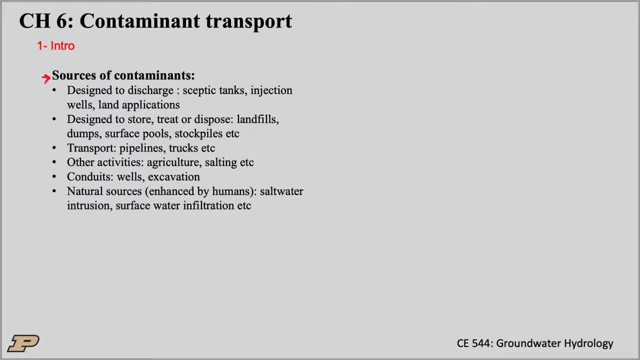 And again, this is from Fetter. This is not from your textbook, but from his Contaminant Hydrogeology, I believe the book is called. So again, I didn't make this list up, I just took it from Fetter. 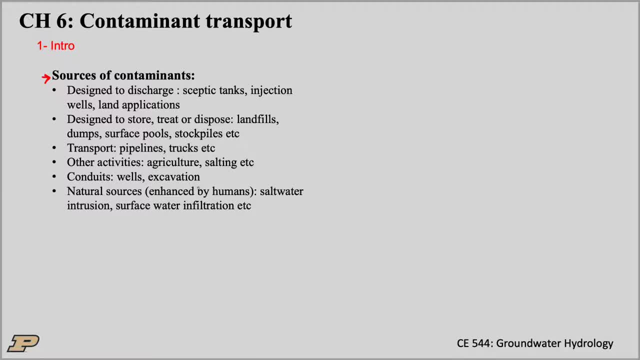 And a lot of the content of these lectures are going to come from Fetter again, as we've done before Again. so the sources of contaminants: right. some of them are designed to discharge contaminants. So let's say septic tanks right, injection wells. 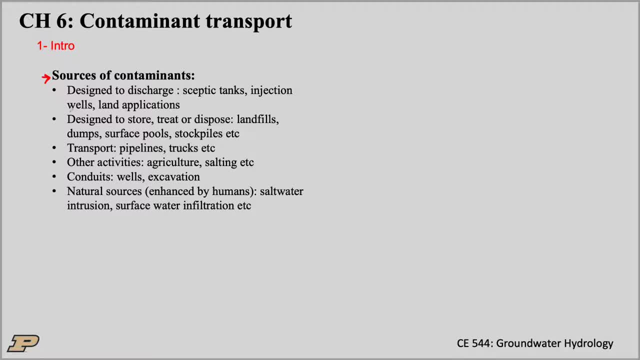 So we use wells, right injection wells, For example, the CO2, right carbon dioxide. Nowadays there's a lot of research on injecting liquefied carbon dioxide back in the earth, basically so it doesn't go into the atmosphere. 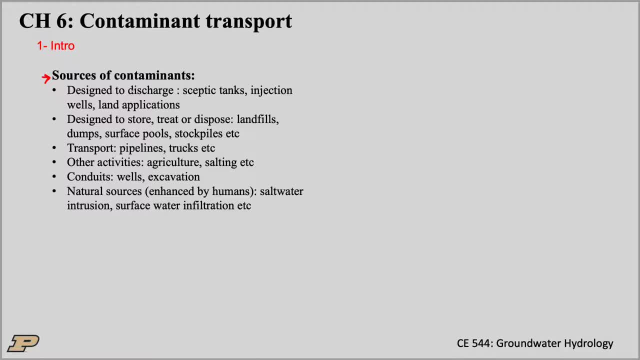 That's an example of you know a system designed to basically discharge contamination, Land application also. So think of, you know, wastewater sludge, for example, that is extracted from your wastewater treatment plant and then applied onto a field. 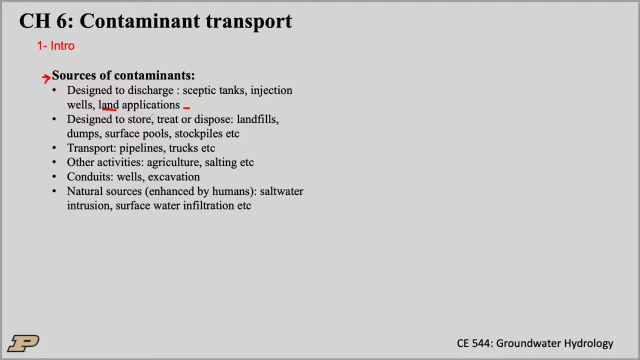 You know, those things usually have a lot of contaminants with them that go directly on the fields. Some sources are designed to store contaminants as opposed to discharge them. So either store, you know, and slash, treat or dispose right. So again, landfills, and we've seen the example here in the GMS illustration. 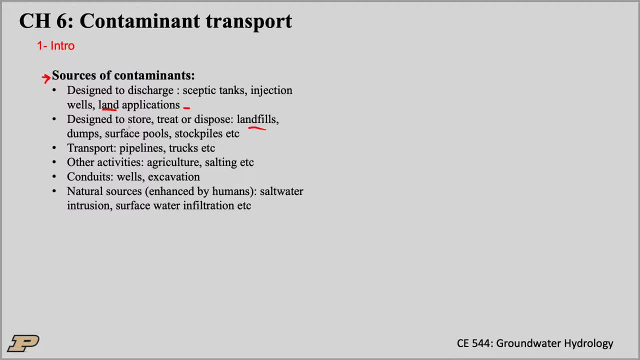 Dumps, obviously, same thing, Surface pools, And these are basically, you know, all your ponds that you'll find in industry To basically store contaminants before it can be treated or released right. So there's a lot of surface storage, basically in ponds, surface ponds that you know may leak into the groundwater. 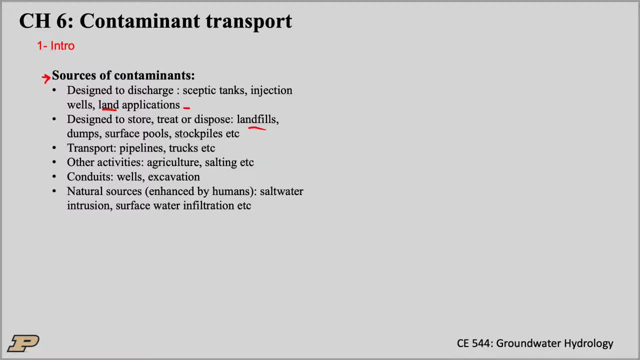 Stockpiles again, I talked about this radioactivity, right, We have stockpiles of uranium, for example, and then if somehow you know there's a leak, then that creates, you know, issues and groundwater contaminations. 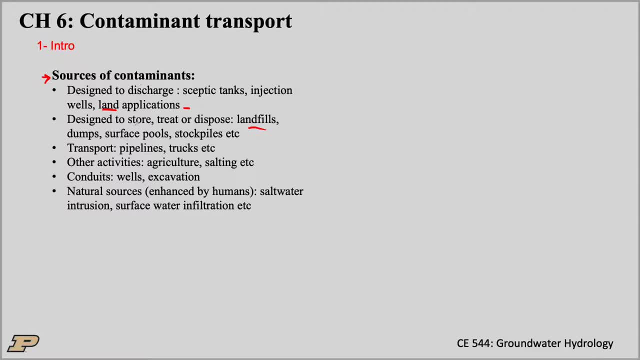 So, beyond the design to discharge or design to store, you know you can also leak during transport. So pipelines are a classic example, right, If you blow a pipeline, then obviously this, you know, whatever it contains is going to leak, eventually down to the groundwater. 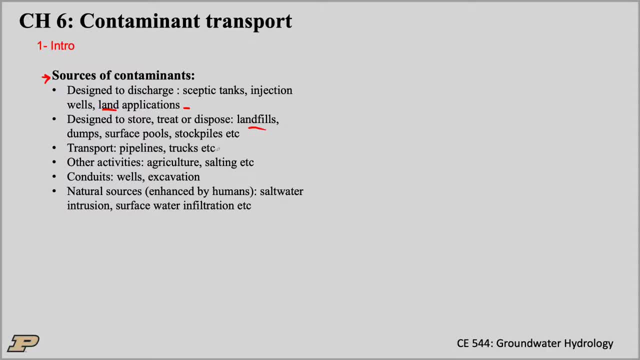 Of course trucks during transport. you know I could put boats and barges here, but obviously those are going to contaminate surface waters first or, you know, slash ocean water, So I didn't put them here, but pipelines and trucks are going to contaminate. 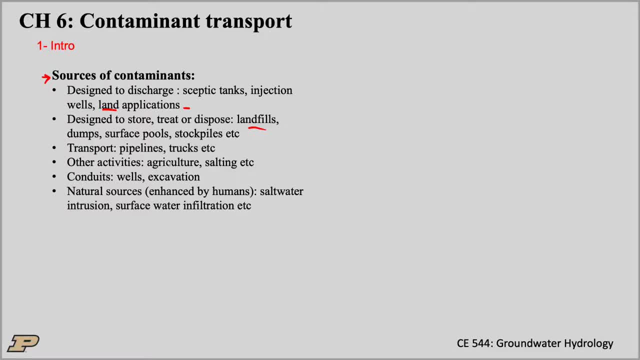 So you know that's one example. So that's one example. Other activities that create potential pollution, even though they're not designed to deal with, you know, contaminants per se. So agriculture is a big one. I do a lot of research on that. 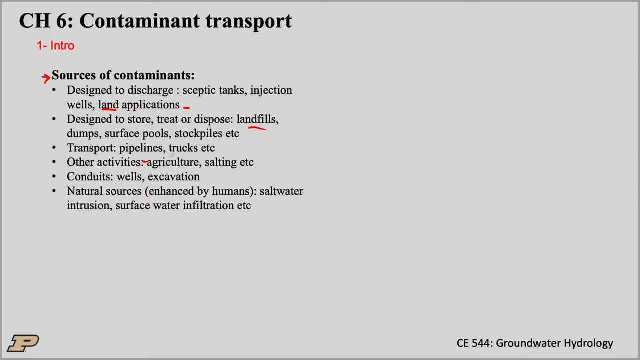 So everything you can think of fertilizers, for example, pesticides, right, that we apply to crops so they can grow better, but, you know, also leach into groundwater supplies and then, you know, create all sorts of problems. 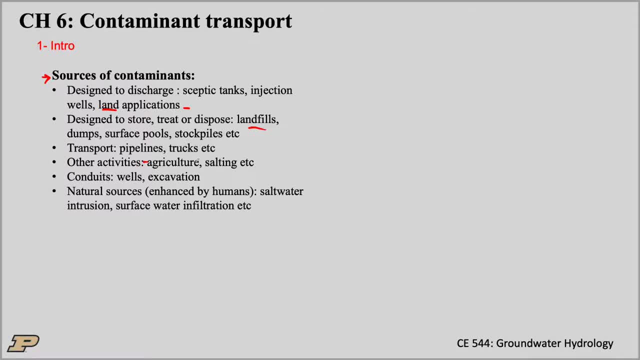 So nitrate, for example, is one. So nitrate at high levels, like we have here, is actually very dangerous for the health. Salting, you know, road salt in the winter is another example you can think of. 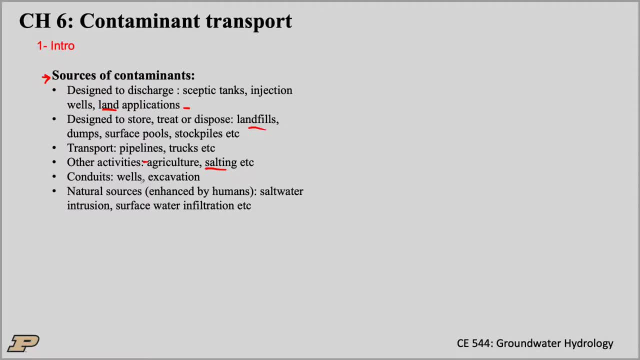 You know we don't put salt to do anything to the groundwater but eventually, you know, it leaks into it. Other conduits, so wells, excavation, are other examples that we've, you know, described a lot during this course. 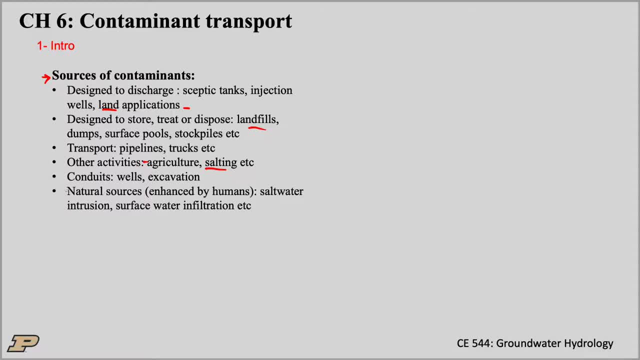 that may, you know, cause accidental pollution, if you will. But you know, saltwater is generally, you know, natural sources, So they can, they may or may not be enhanced by human activities. But for example, saltwater intrusion, you know, on coastal aquifers. 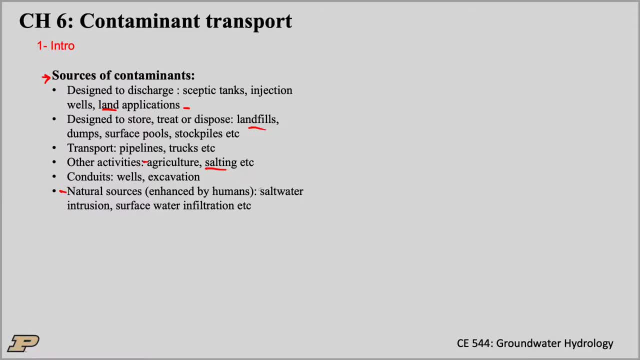 So if you have pumping near the ocean, you know you're actually increasing saltwater intrusion, right? Because if you're pumping the freshwater near the ocean, obviously the void left is going to be filled by that saltwater. And then you have salting of all your coastal aquifers, which is a big issue. 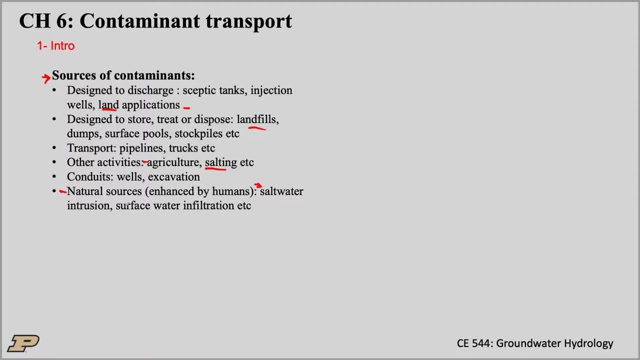 Both environmental and also for drinking water, because of course you don't want to pump saltwater. Surface water infiltration- again, this is a broad category here, But if you have, you know, a wetland or a lake that is connected to your aquifer. 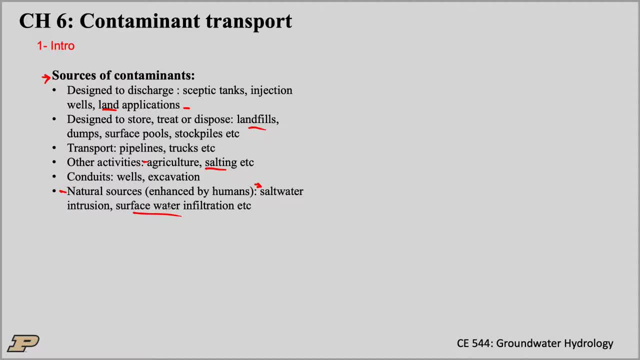 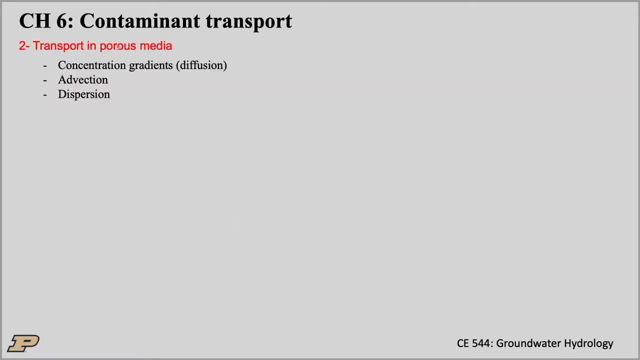 and then, if that wetland or lake becomes polluted for some reason, right, this infiltration, which is natural, will cause the pollution of your groundwater. So a lot of sources of contamination, potential contamination. Okay, so let's get into the core of this lecture, which is the transport itself. 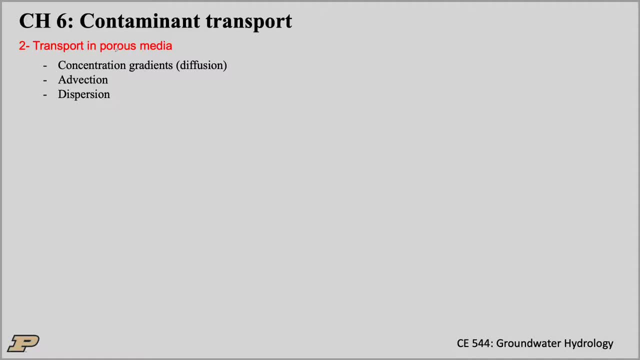 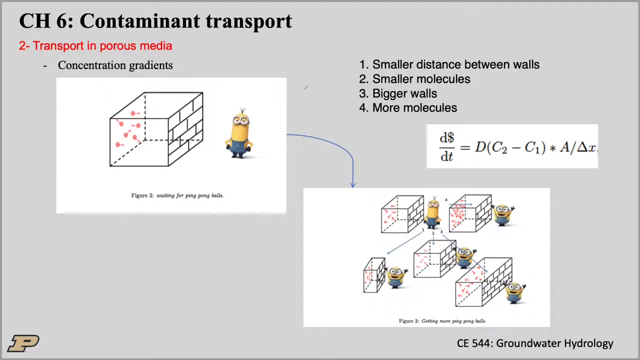 So this was a broad introduction on contamination And now I'm moving on to actually describing the processes and equations that describe those processes of the transport. How do things move right? How do these contaminants move in the groundwater? So the first case I'll describe, and some of you will recognize that from my 547 course. 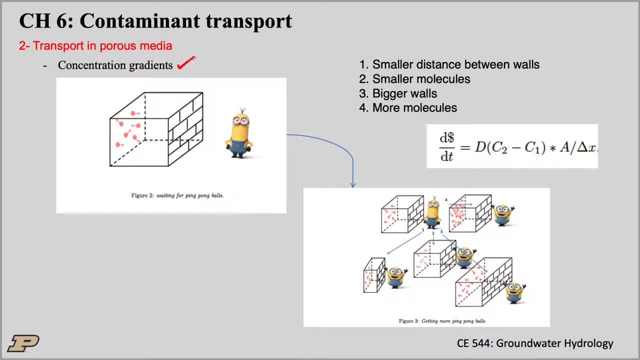 the first process right is just concentration gradient. So even if the water doesn't move, if there's no movement of water itself, right? if you have pollution somewhere, it will move just by concentration gradients, right? So if you have a lot of something somewhere, right? 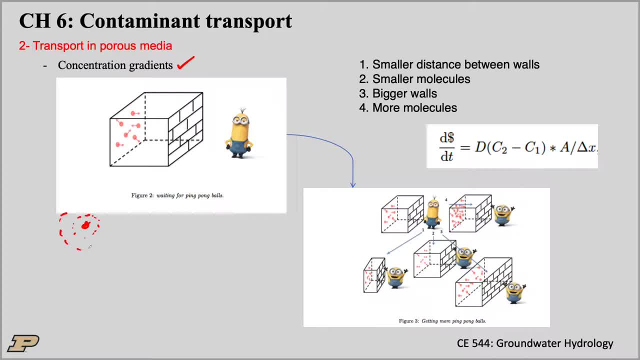 just diffusion will increase its influence, you know, over time. So how does that work? Well, there's basically four aspects, right? So this is a little game. You can think of this So conceptually, right, if you remember this little picture. 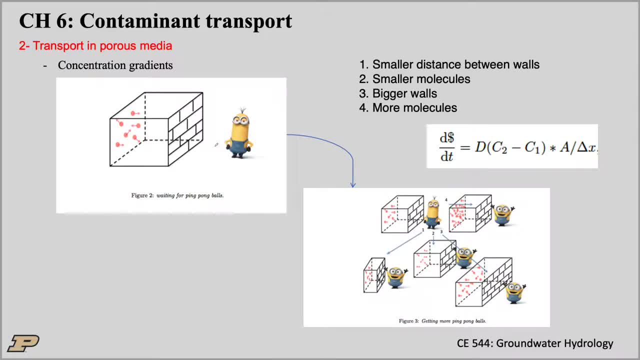 you can backcalculate or backtrack the process that influenced diffusion. And those are the smaller distance between the two walls right. So the closer you are from the source right, the more those particles. if you imagine, those are little molecules, right? 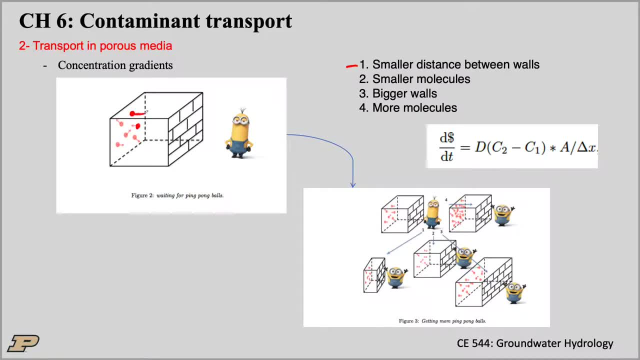 those little balls here or dollars. you know, the closer from the source you are, the more of them are going to reach you right? Smaller molecules, right? So if they're like tiny molecules, they can move faster. if you will, they diffuse faster. 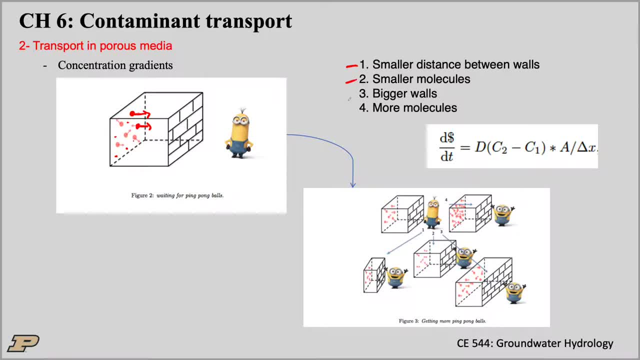 So the smaller they are, the faster they will diffuse, Of course, the area of the wall right. So if you're collecting, you know, from here, versus if you're collecting from the whole surface area, obviously you'll have more of them, you know. 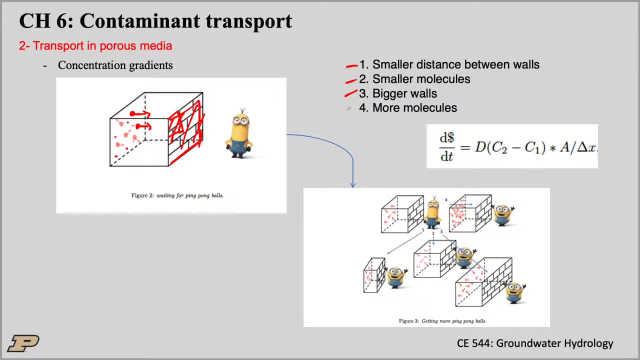 so it depends on the surface area, the amount you collect And of course, the concentration. I already mentioned that, but you know, the more you have to begin with right. So the concentration gradient, the original concentration. 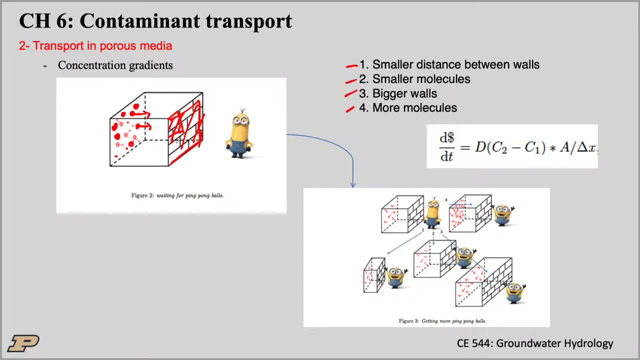 the more you have to begin with, you know, the more you will receive at whatever observation. well, if you will, observation distance you're at Now, if you put those things together right, you can see here I put a dollar sign. 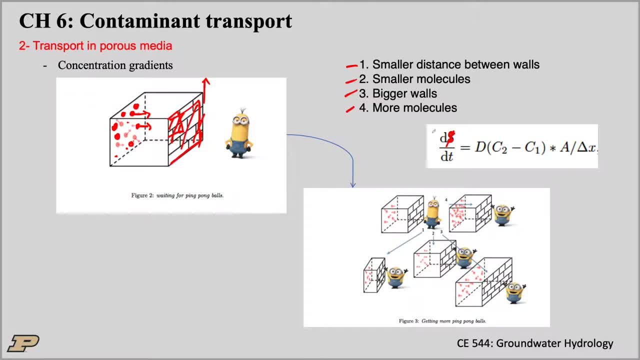 so imagine these were dollars. you want to maximize your amount. That will depend on the diffusion coefficient, which is essentially the size of the particles. right here, number two. right Then the concentration, so number four, the concentration gradient, really. 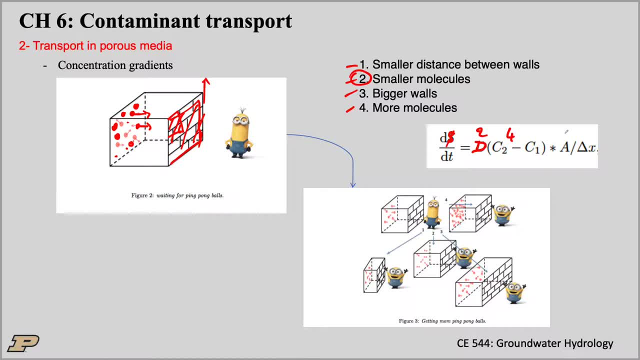 but the concentration itself, right, is what drives the flux, The area of the wall you collect at. so that's number three here. And then the distance right between you know, the observation to your distance which is right here. one: 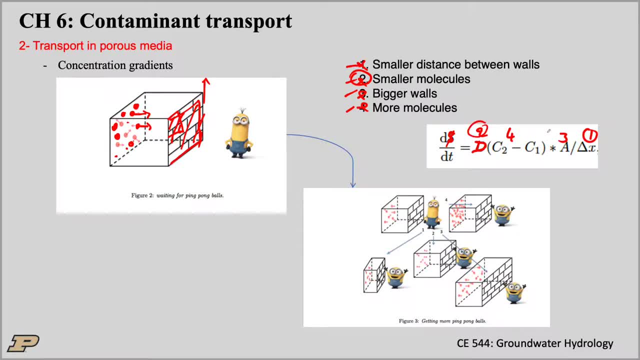 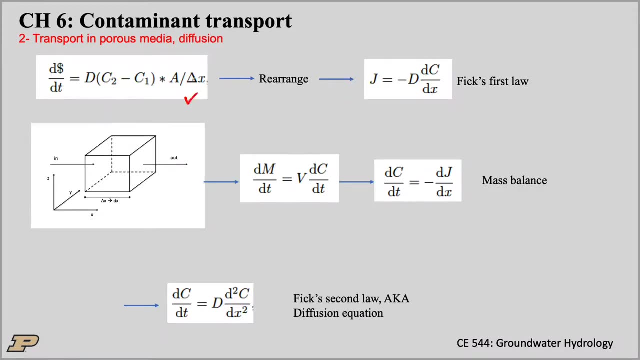 Yes, so one, two, three, four, You have four different variables that influence the amount per time of molecules we get. okay Now. so again, I just repeat this equation here. You can see that it's proportional to the size. 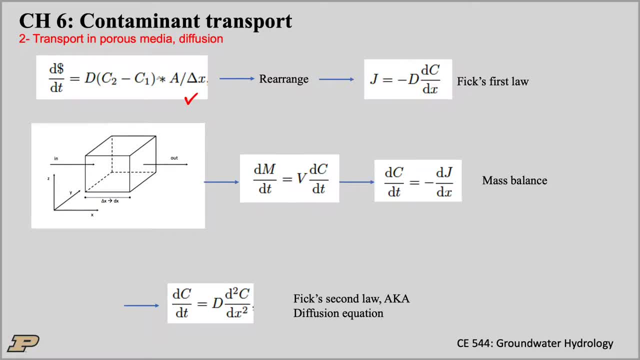 of the diffusion coefficient proportional to the concentration gradient, proportional to the area and, inversely, proportional to the distance of the observation to the source. Now we can rearrange this equation to express it as a flux, right? So you can see that again. diffusion here is here. 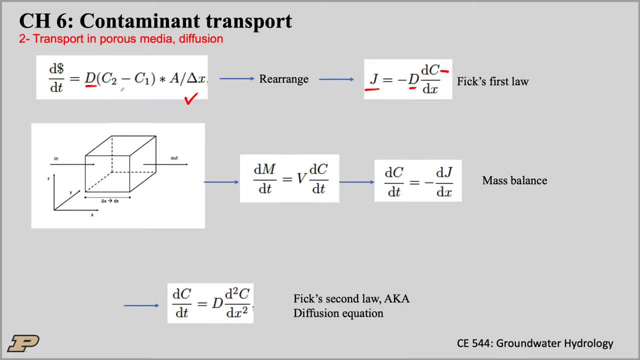 the concentration gradient is here, right, dx is here, So now we're missing a, So j, the flux here that I call j is, you know, the amount per area per time, right? So it's like some mass. 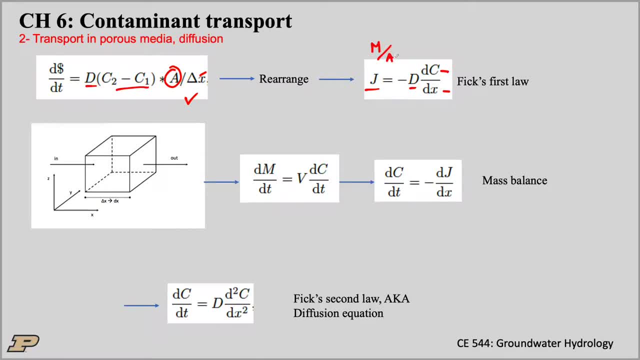 or some number of particles per area per time. That's your flux. okay, So this is Fick's first law, and it just states that the flux is proportional to the diffusion coefficient and the concentration gradient in space. okay, Fick's first law. 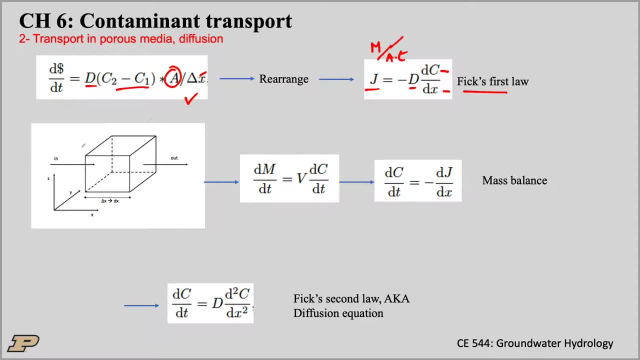 Now, if we express a mass balance. So again, mass balance is just, you know, whatever comes in must either come out or be disappeared inside the volume, right? So if there's mass in, it can stay in the volume. 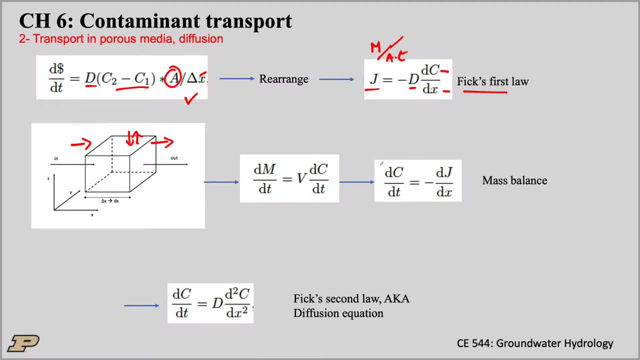 so there's more mass in the volume or it can come out. This is just a statement of mass balance. So the change of mass per time is, you know, the volume times the change in concentration, And we can again rearrange that as. 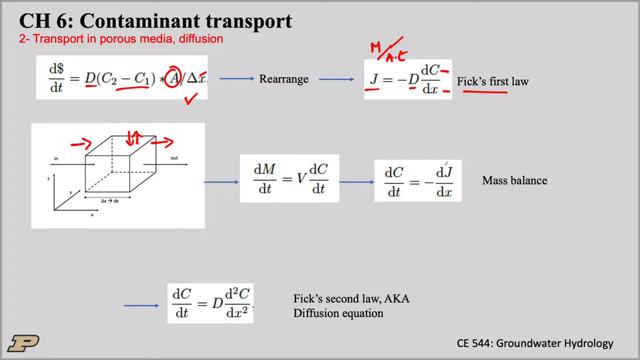 the change of concentration per time is the minus, the change of flux per distance, right, It's flux in, flux out. So this is just statements of simple statements of mass balances. If we combine, if we carry that calculation right. 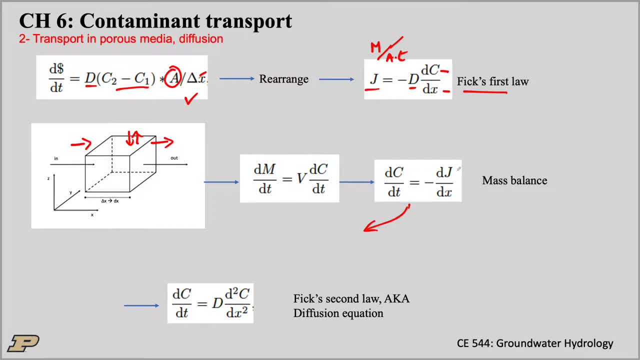 So minus d, dx of the flux right, You can replace the flux here by its, by its value, by the diffusion times, the concentration gradient right. So if we replace j by d, dc, dx, you can see that now we have the second derivative right. 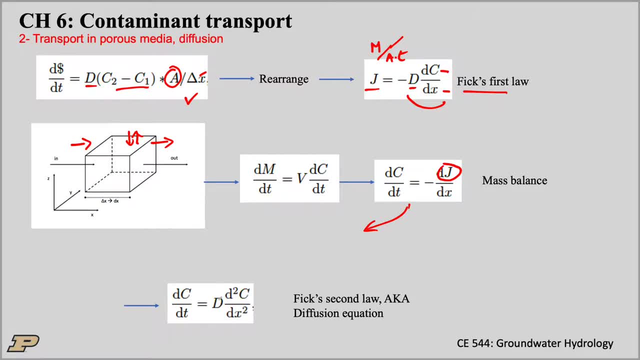 d, dx, d, dx, that's d squared over dx squared c, and then the diffusion is here. Note that minus and minus cancel. so now we have a plus sign here. So now the change of concentration over time in that control volume, if you will. 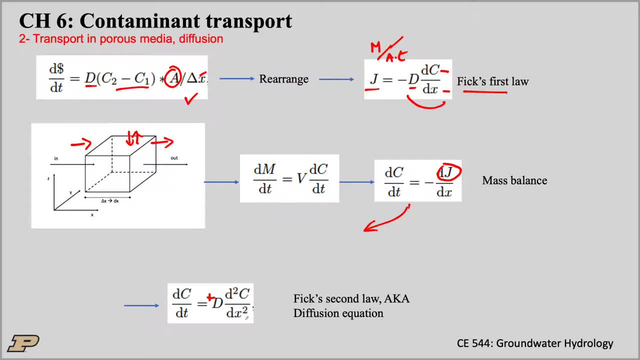 is the diffusion coefficient times, the second derivative of the concentration, the second spatial derivative of the concentration, which is Fick's second law right, And this is also known as the diffusion equation. Okay, so this is how you derive the diffusion equation, basically. 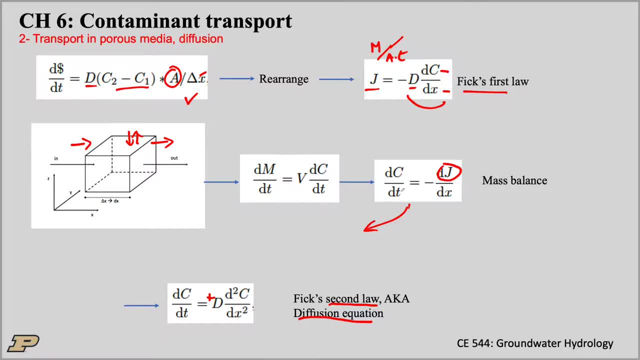 Start with the ping-pong balls, or you know the little Minion cartoon. Remember those four variables that influence, you know, the change of molecules reaching that observation observer per time, and then you can, you know, work that out. 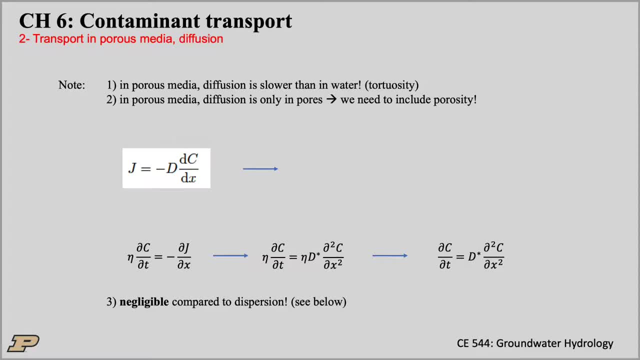 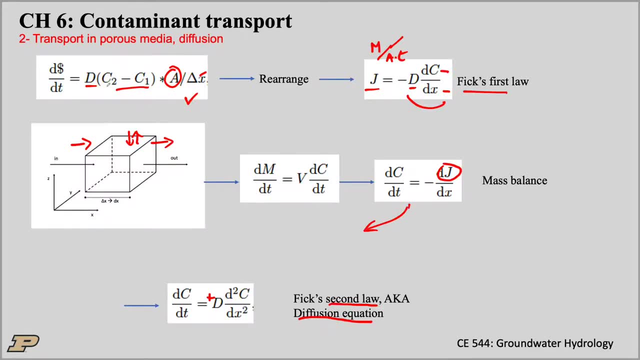 Okay, So a couple notes here to conclude on diffusion, So in porous media. so this was all a general- sorry, a general- derivation right of the control volume that is filled with water. Now in porous media, the problem again. 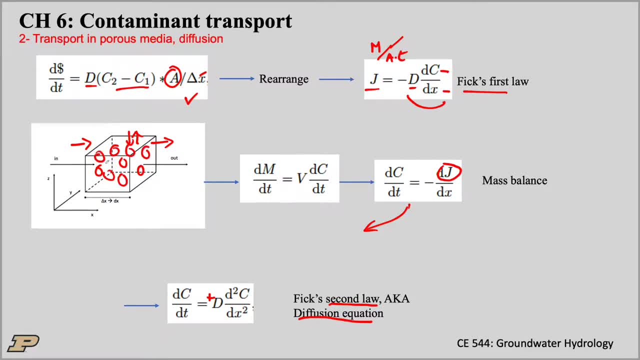 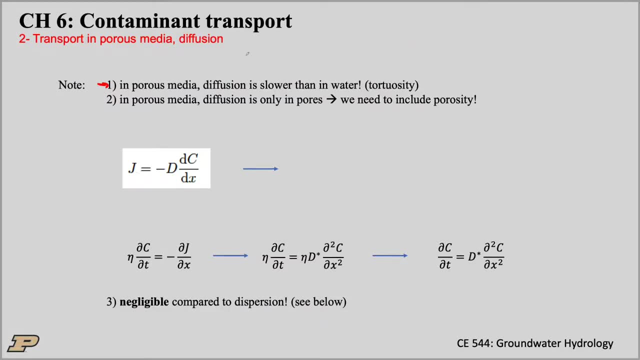 we have well solid particles and we have water in between right, So that creates a couple of complications that we need to note here. So the diffusion is slower in porous media than in water, And that's again because now we have particles. 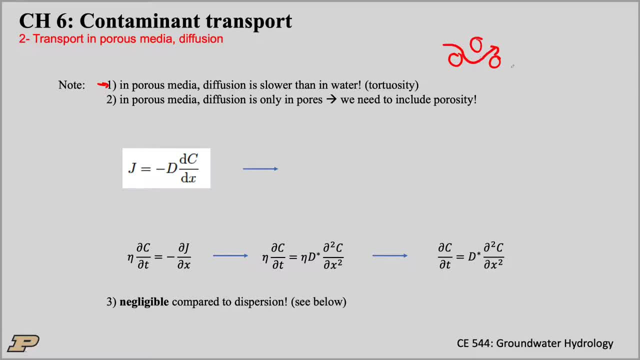 so now the molecules diffusing have to go sort of that contorted flow path, right? So if you have a molecule diffusing here, it can diffuse through that solid grain here. so it has to go around it so it diffuses slower, right? 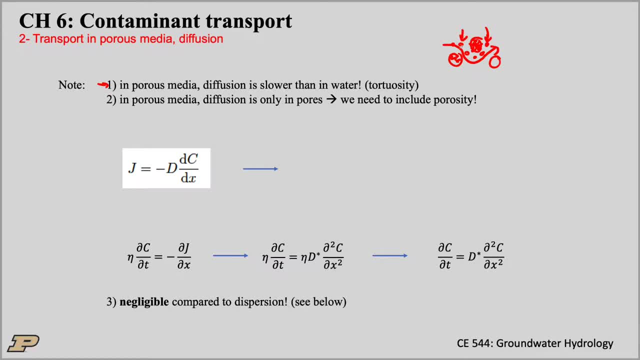 The time to reach this position down here from here right is longer because it had to take that contour right. So this is called tortuosity, Also in porous media. obviously the diffusion only is in porous. So this is similar but not exactly the same right. 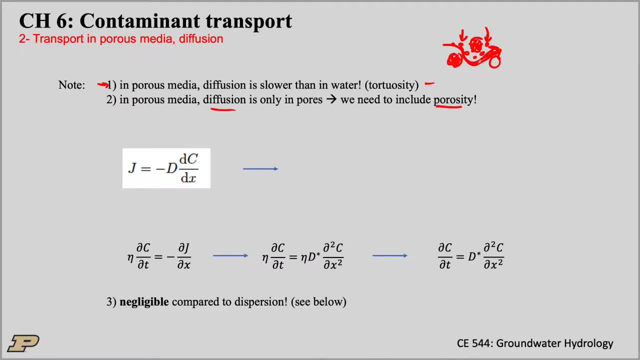 Because the fact that there is porosity means that diffusion will only happen in a portion of the volume. right, If you have total volume here? right, the diffusion only happens in the liquid phase, so we have to include porosity somehow, okay. 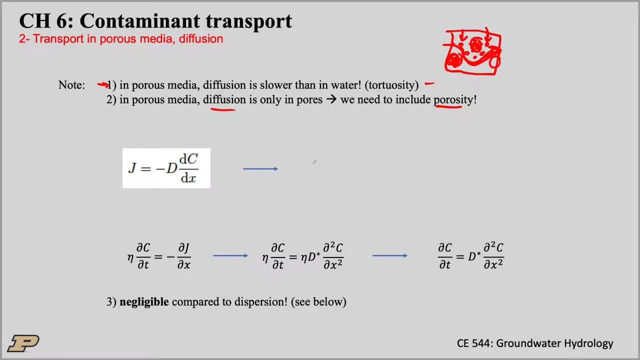 So now the flux, instead of just being minus d, dc, dx, actually is minus d star, which is that corrected diffusion coefficient for tortuosity, right. So if you take the diffusion coefficient of, you know, any molecule in water, 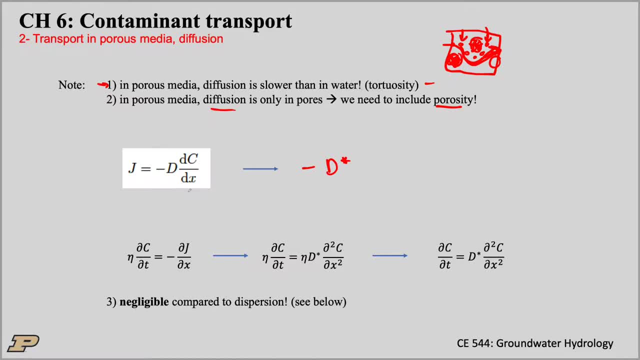 let's say salt in water, you get a number Well in groundwater, right in a porous media. now you have to modify that diffusion coefficient for tortuosity so it's actually less, And again, because it's only in porous. 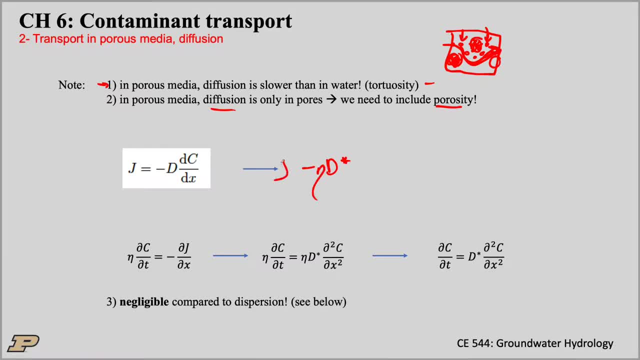 you have to include porosity. So really the flux now becomes J equals minus eta, again the porosity same nomenclature as before. So this modified diffusion coefficient for the porous media times: dc, dx. Okay, so this is really the equation. 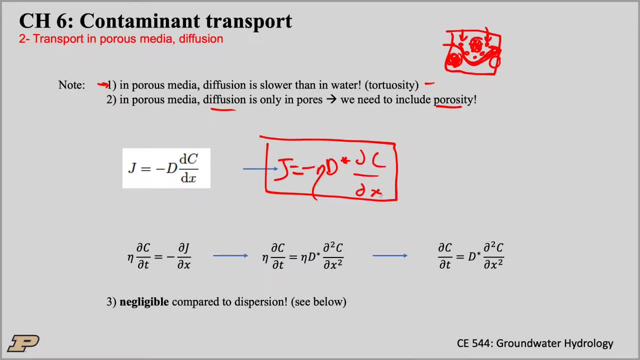 we work with for groundwater. That's the difference between the groundwater and just diffusion in water. Now if we calculate again the derivative of the flux, the special derivative of the flux right that mass balance equation, again we have to include 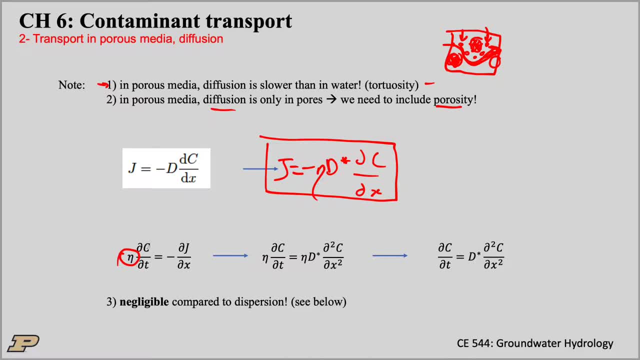 this porosity term. So really, the change of concentration per time in the entire control volume must include porosity, right? So the porosity times the change over time. is this equation right? So now, if we rewrite the whole thing, 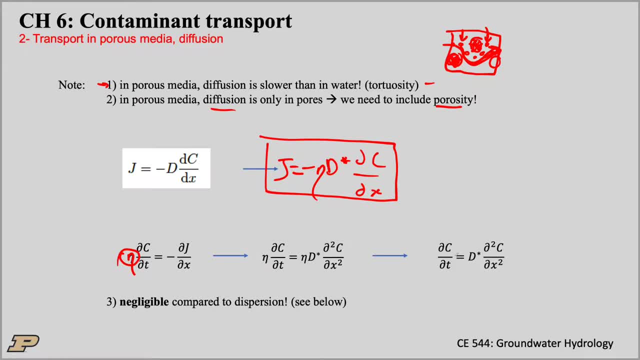 you can see, porosity is on both sides, so that will actually disappear, And then the change of concentration over time will be that modified diffusion coefficient for tortuosity times, the second derivative. So we end up with a similar equation than the one. 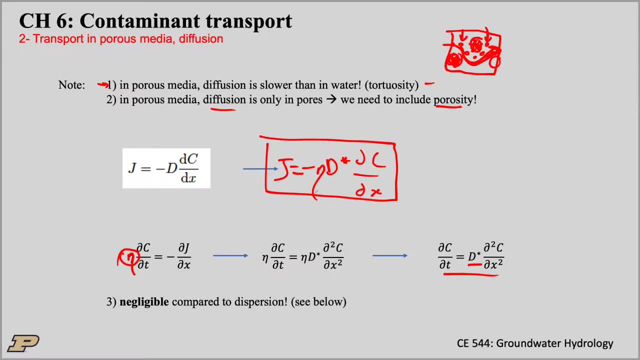 for just water. And again, that's because for the flux you have to include the porosity, and then you have to include the porosity for the change over time, So they end up canceling and you just have the tortuosity. 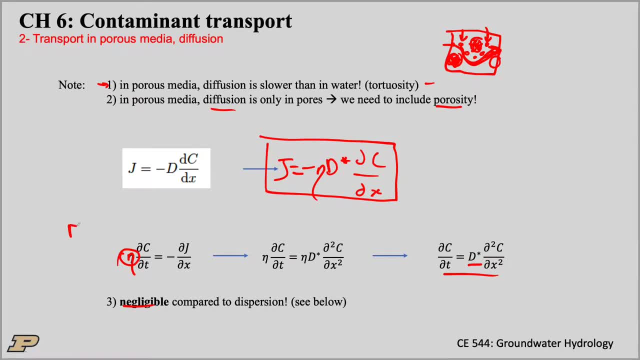 that remains Now a final note for the diffusion, and diffusion only meaning the concentration gradient, transport. this is actually negligible compared to dispersion, And again we'll see dispersion, but remember that diffusion is usually very small compared to actual transport. 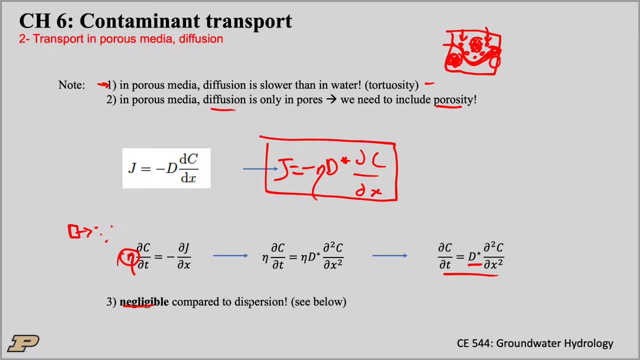 So when there's velocity, which we'll see right now, then the velocity differences in the porous media creates some dispersion- And again I will define this in a couple slides- And that dispersion sort of overwhelms the diffusion. typically, 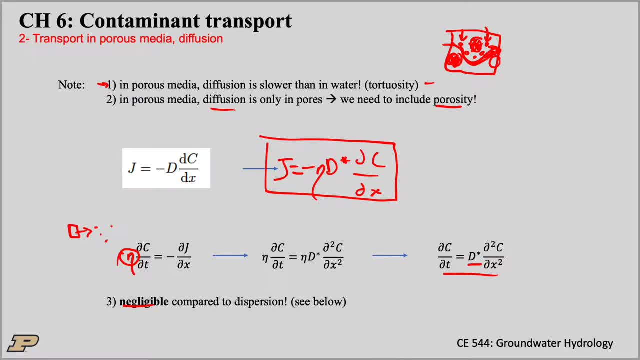 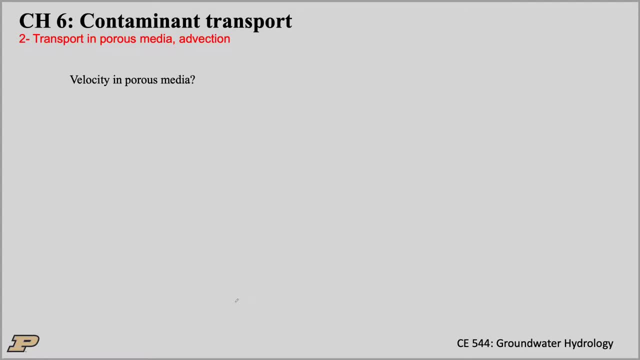 So diffusion is usually not a very important process, but the duration I just did is the same for dispersion. So it's really important to understand those fluxes and how that works, basically, Okay. well, how about advection right? 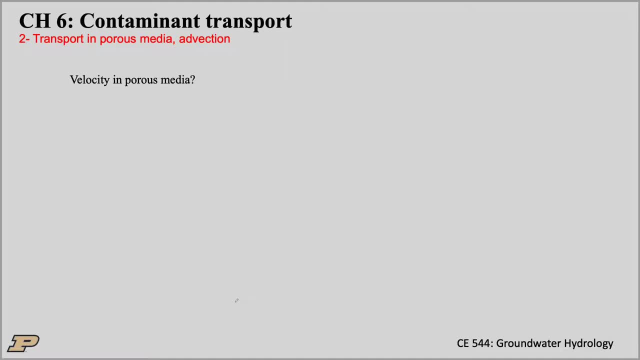 So advection is transport due to velocity, And we've seen velocity in porous media before right in this class, So we've talked about this over and over. What is velocity in porous media? Well, you'll remember that is. 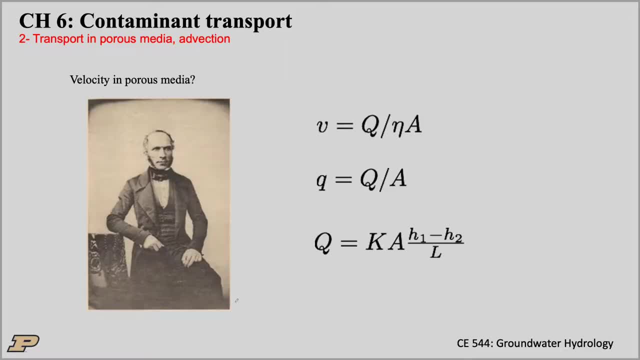 the Darcy flux divided by porosity. right, We've done this over and over Again, that old picture of Darcy, and just again reminders of, you know, previous chapters. that's chapter 2, where the velocity of the water. 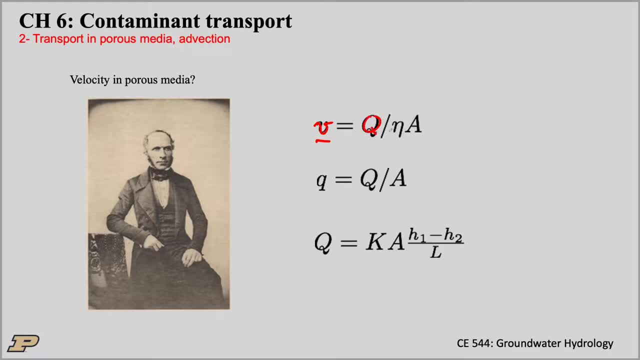 of the groundwater, of the porous media water is the Q, the discharge right in volume per time, divided by again the porosity times, the area right, This is the actual velocity of the flow coming out of a column of porous media. 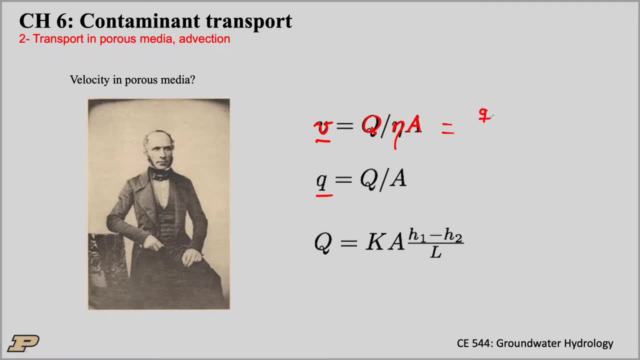 Now you'll remember that Q over A equals Q over eta, right, We've seen this over and over and over. But this is the velocity. we're talking about the actual velocity of the water, not the normalized flux, not the Darcy flux. 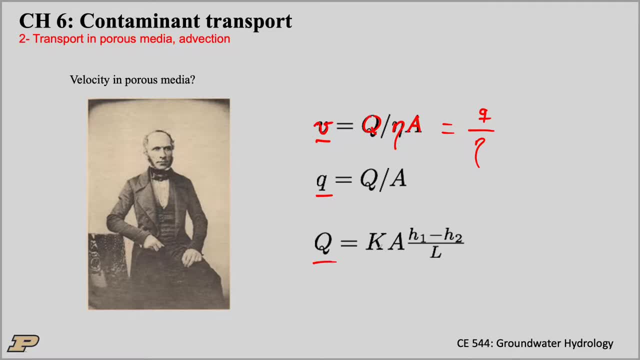 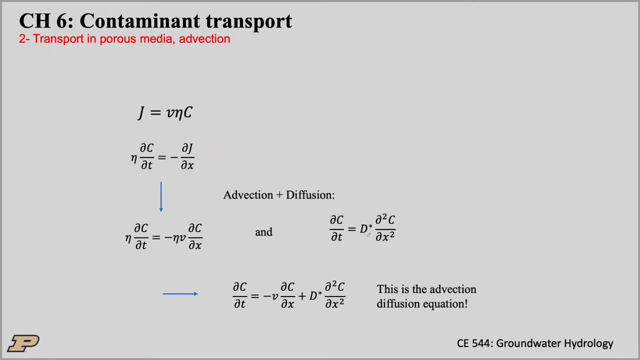 And then, finally, because we know the Darcy flux, we can replace everything in the equation right and have: Q equals. you know the k, dH, dx, which is the Darcy flux times A. Okay, now if we go back, 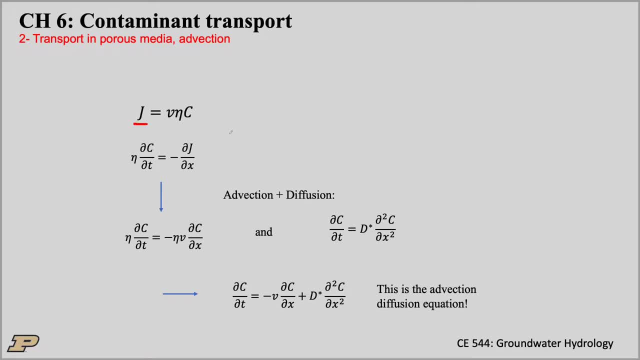 to writing it as a flux, right. so now we're interested in those scalar or in those masses or mass of contaminant quantities. so the flux of contaminant due to advection, again V here is the velocity, so the flux is the advection. 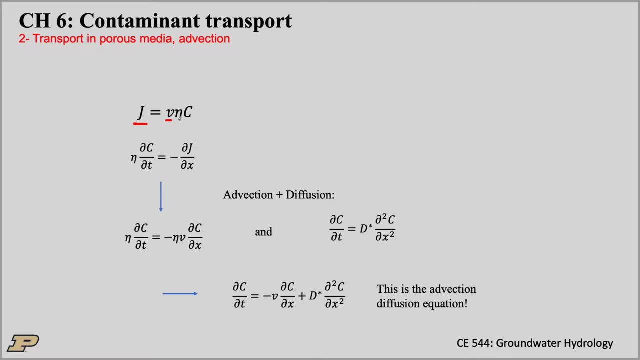 the velocity of the water times the porosity. right again, because there's only in the flowing water that things move. the flux is the advection. so this is your advective flux. Now again, like before, right, the change of concentration. 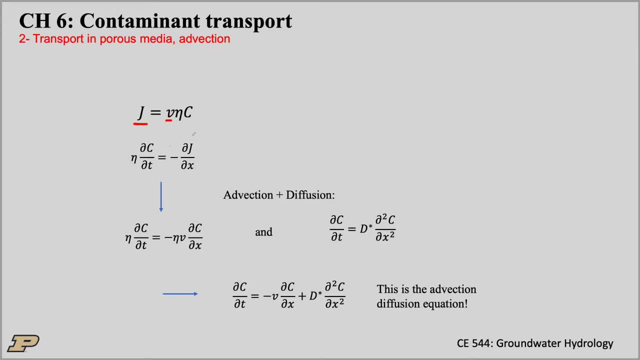 over time in a control volume or somewhere, is the first derivative of the flux. so it's exactly the same, you know, as we did before for the diffusion, Now we replace this. now this flux is the advective flux and not the diffusive flux. 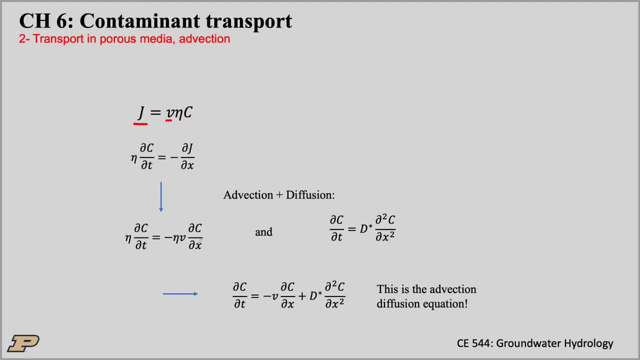 so we replace with this value dcdx. okay, so now V eta c, V eta c and then the ddx- ddx. so everything is consistent right. Once again, you can see that the porosity appears on both sides. 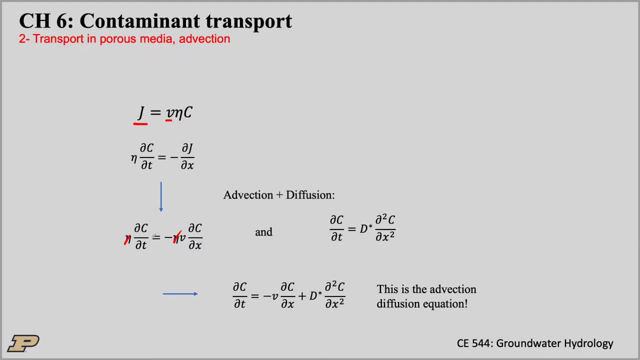 so we don't need it anymore and we find that the change of concentration over time due to advection equals, minus the velocity times, the concentration gradient. okay, and then finally, we're arriving at our goal here, to put the advection and diffusion together, right? 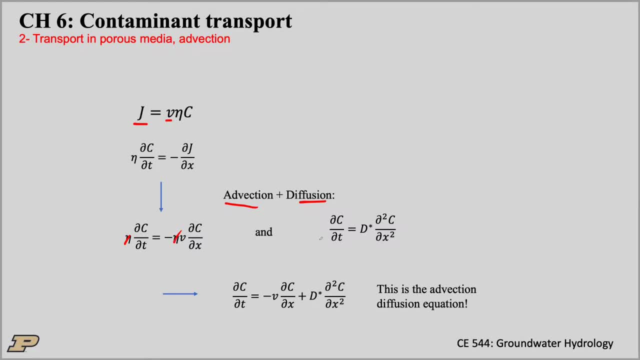 so we have this left side left hand side term for the velocity, this right hand side term for the diffusion that we've seen before. now we can put them together right. so we have dcdt equals minus V, dcdx right. 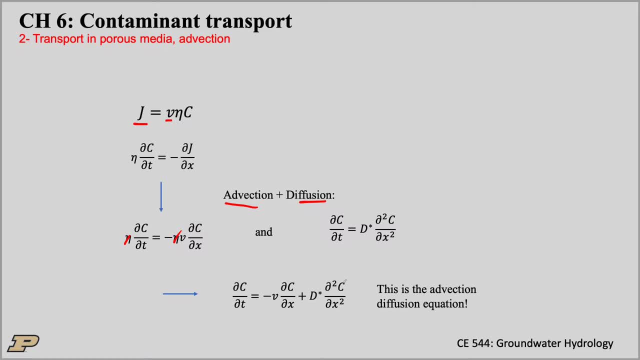 the advective flux plus the diffusive flux. so d star again. and the second derivative of concentration, And this is your advection diffusion equation, This is your transport equation that we'll use over and over for this chapter. Okay, finally, what is dispersion? 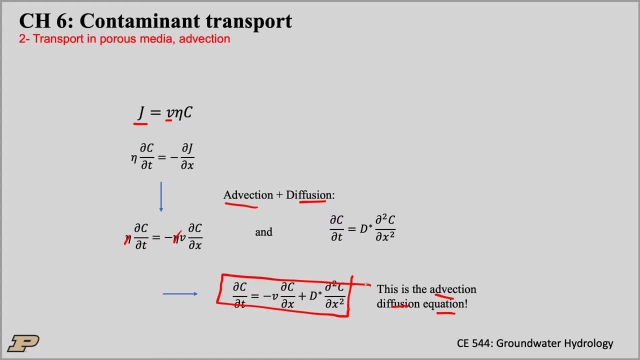 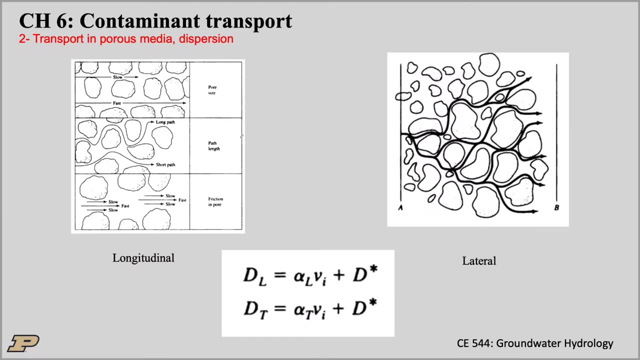 So I said before, diffusion is negligible compared to dispersion. Well, what is dispersion? Oops, excuse me. So here's a definition, or an illustration, I should say, of what dispersion actually is. And again, these figures are from Theder. 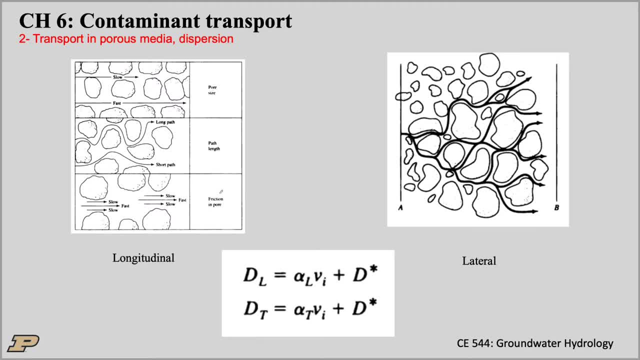 There's like basically three different mechanisms that create dispersion. The first one is the pore size, right, so you can see that here we have a macro pore that creates fast velocities or lots of flux here, and then maybe some smaller pore where the velocity is much smaller. 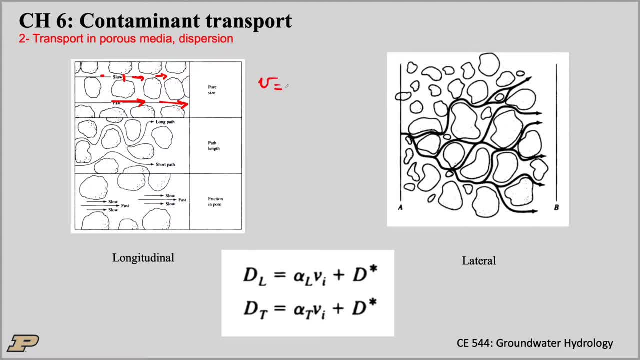 So if you have fast and slow velocity now, V is not a constant right, there's different velocities at different places, so that the particle that starts here will arrive here much faster or much before the particle that starts here and will take, you know. 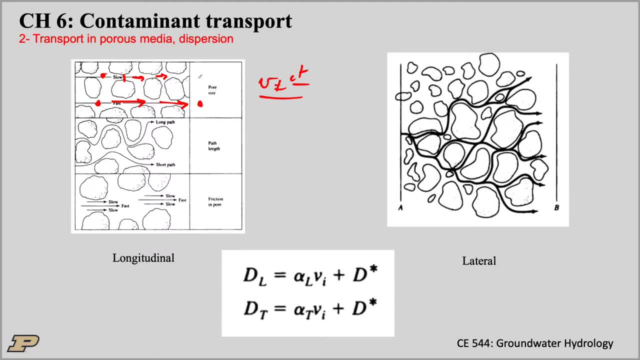 a long, long, long, long time to get to the same point. So those you know at the end here we get particles that are spread out in time, And that's basically what diffusion does, right? So it's the same as diffusion. 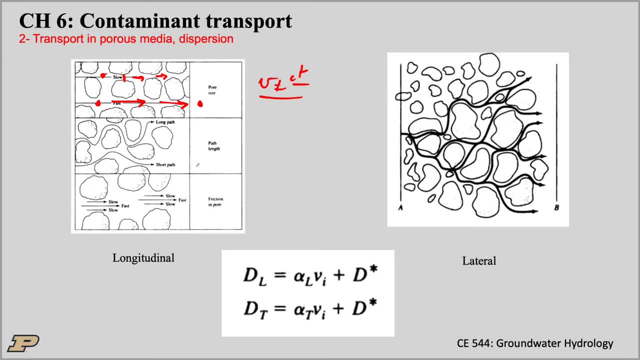 but now it's due not to consumption gradient but to velocity gradients, if you will. right. So now, this is the influence of velocity gradients. Now, similarly right, if you have a flow path that is much longer right, it will arrive much later. 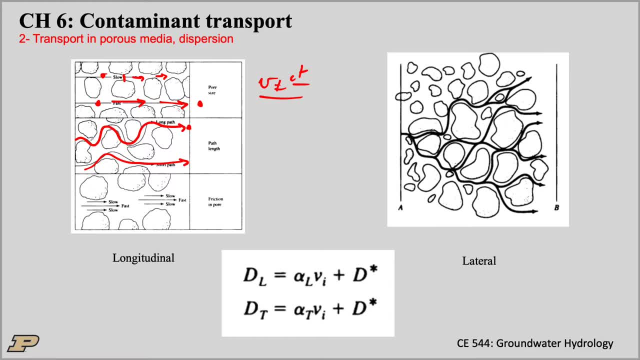 than this particle here, just because it had to go again. that's like the tortuosity story, right? It had to go around and around and around for a long time, whereas this guy had a much straighter path. so again, this guy is going to arrive first. 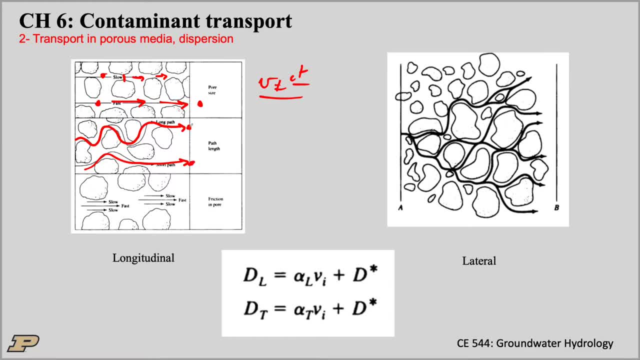 and the top particle will arrive much later. so now we have a spread in time again of that arrival times and that's basically a definition of dispersion, And then finally just within pores. you'll remember we've done that again in number three. 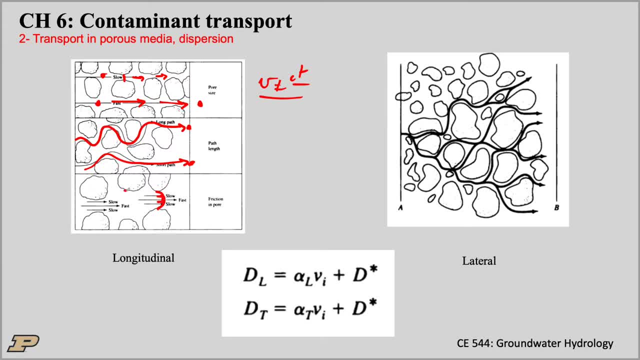 like those sort of Poiseuille flow within pores, right where you have those velocity distributions with fast velocities in the middle and basically no slip conditions right at the grain interface. right there's like basically zero velocity to very fast in the middle. 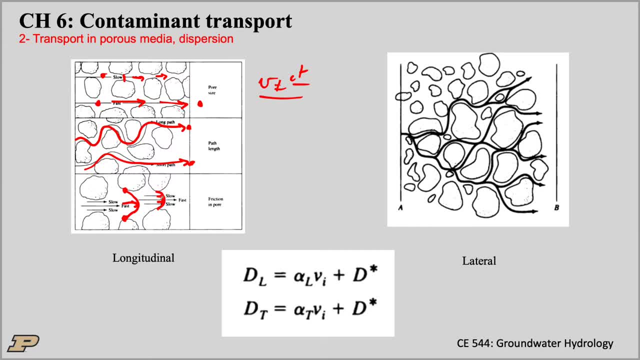 so again, velocity distribution, which creates then arrival time distributions, which creates then an influence on dcdt right. If the time changes, then you know this term is affected. So this is what influences longitudinal right arrival times, if you will. 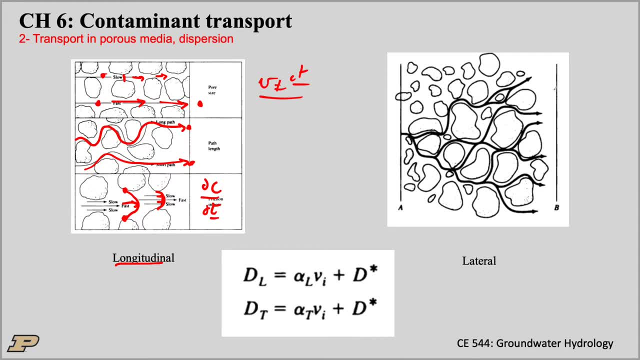 or how fast things get to a point. Now. the same thing is true on the lateral side right. So if you think of this as a top view, you can see that if we all start at that same point, just because, again, of tortuosity, 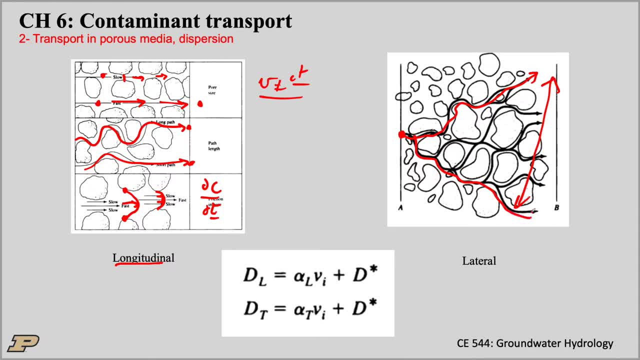 things are going to spread in that second dimension, right, let's say this is y and this is x, right, So this was all in x here we didn't consider any y. so here in y, you can see there's a spread. 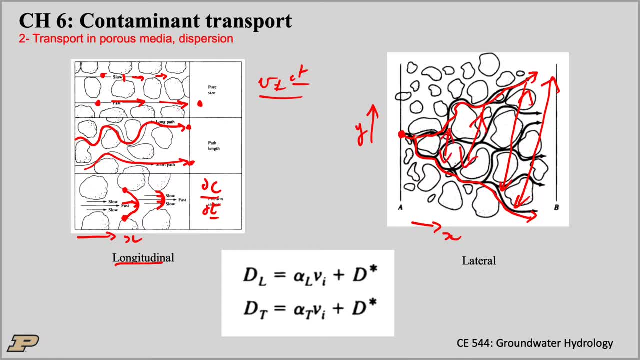 of the plume. that is due to that second dimension, if you will, dispersion, tortuosity. So things go up, things go down and depending on where you end up, it's going to be in the lateral direction. So we can put those two things. 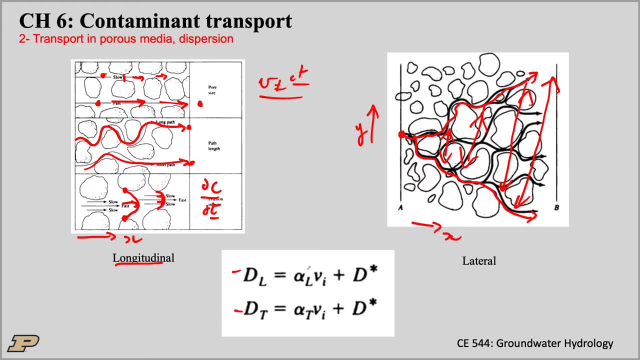 you know, in those expressions. So basically we've seen that dispersion is due to a distribution of velocities. So we can see that in the longitudinal, in the longitudinal, dispersion is proportional to some longitudinal dispersivity or a coefficient- here alpha. 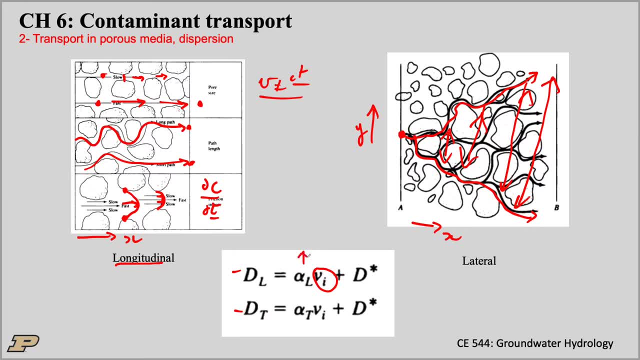 times the velocity, And you can see that alpha is the length, dimensions of length. So velocity of course is length per time. Dispersion is like a diffusion coefficient where it's length squared per time. So alpha L here. 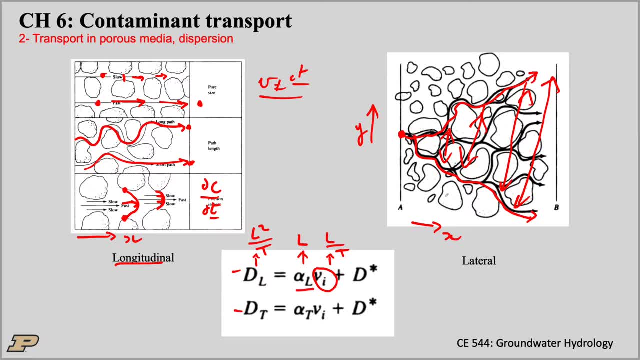 is length, scale and typically it's related to the grain size right or the distribution of grain. so I won't go into that too much, but you can see how this works. And again, plus d star, this is a diffusion coefficient. 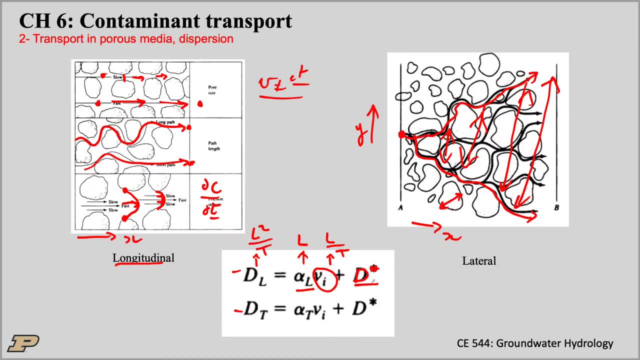 Now what I've said before, and this is where you can see how the diffusion coefficient here usually is orders of magnitude less than the dispersion coefficient here, so that the overall dispersion coefficient- hydromechanical dispersion- is essentially just alpha.